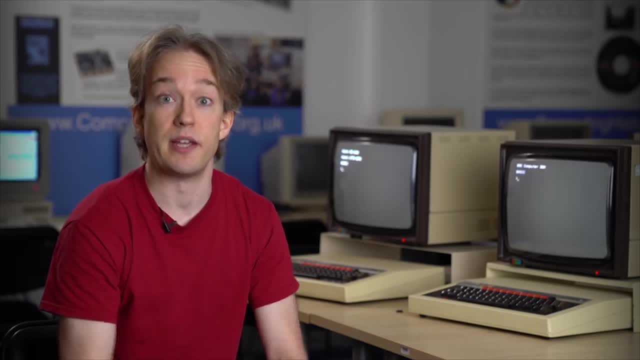 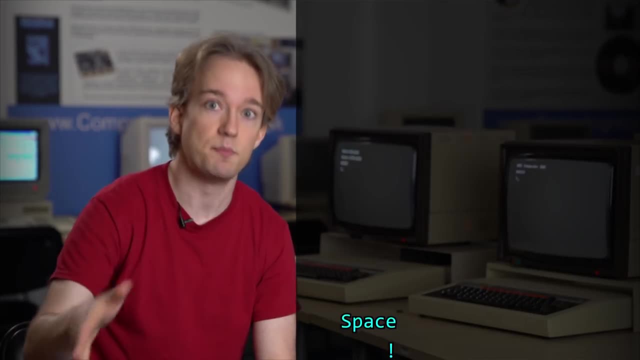 that it gets more complicated than this, but hey, this series is called The Basics, so deal with it. On a modern computer, each English character takes up exactly eight ones and zeros on disc, Eight bits or one byte, And there are 256 possible combinations of those ones and zeros. 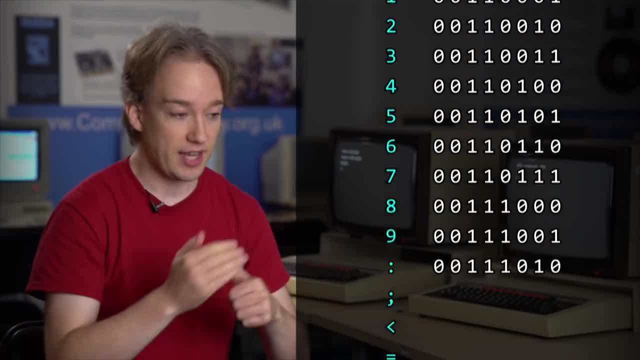 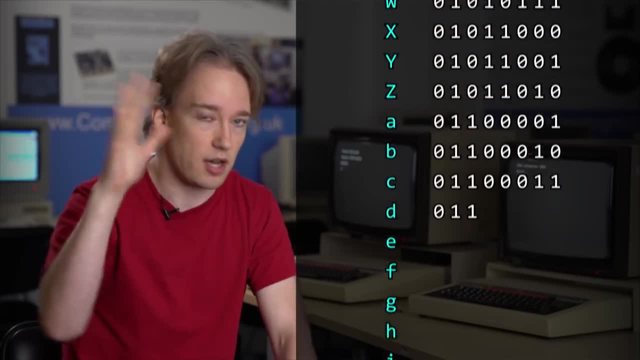 so you can have 256 possible characters. That's enough for the English alphabet numbers, some punctuation and Well. then it gets complicated depending on which country you're in, And oh my god, that's a whole separate video we do not want to get into right now. Why eight bits? Because it was big enough to store all the characters that American computers usually needed, but no bigger, so the text doesn't take up any more space than it absolutely has to. Eight is also a power of two, which means it's easy to deal with at the really low levels. 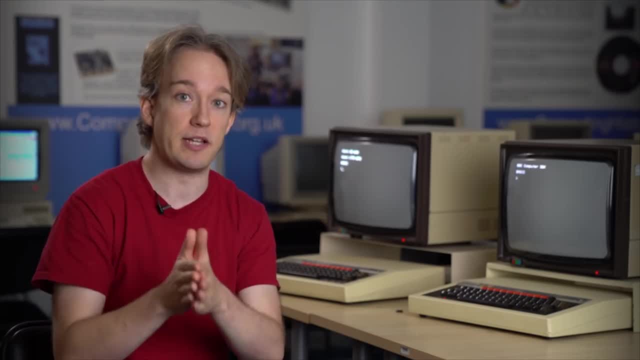 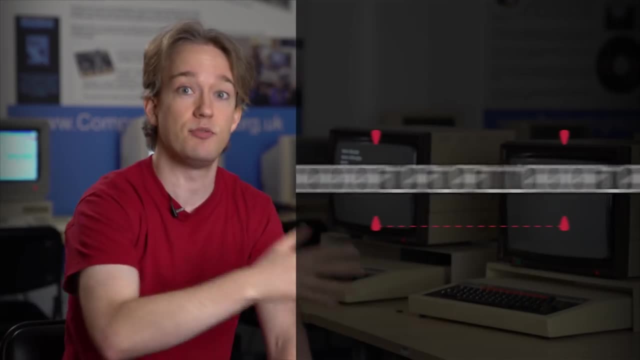 of programming. It's also helpful to have a fixed number of bits per character because it makes searching through text really fast. If you want to go to the 100,000th character in some text, you know exactly where the ones and zeros are going to be. 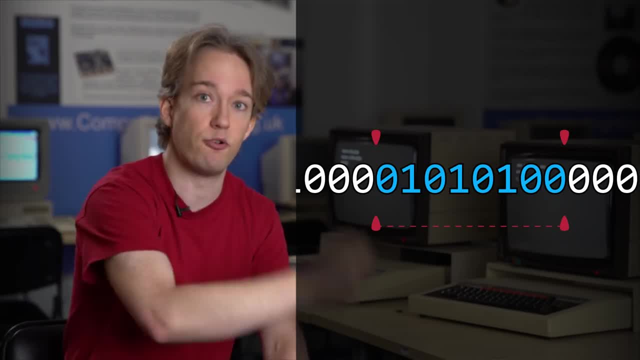 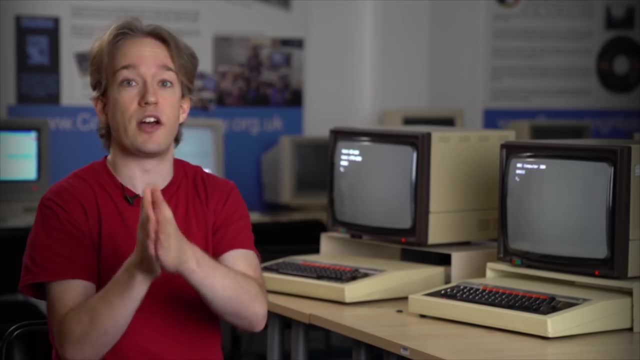 without having to count the number of bits in every single character before it. If you want to know how long a string of text is, you just count the bits and you divide by eight. Computers don't have the luxury of spaces, remember. It's just one long string of ones and zeros. 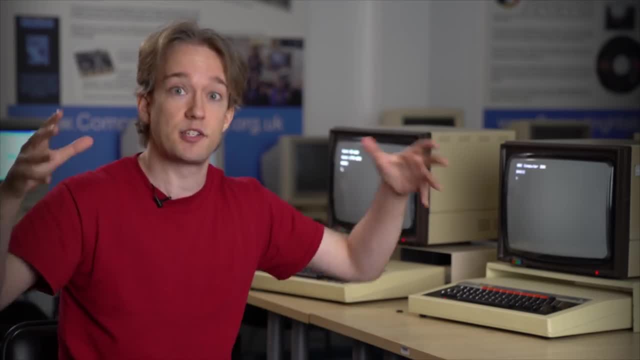 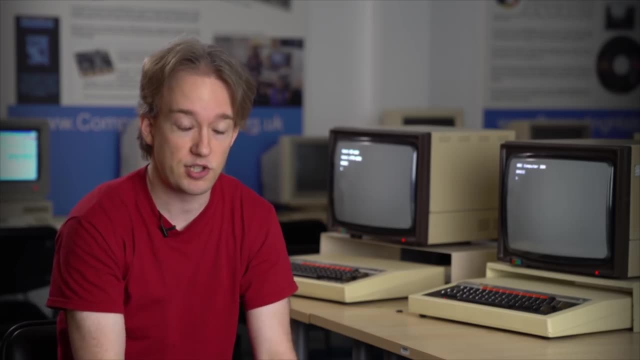 But let's say we're not worried about speed right now. We just want to fit as much text as possible into a smaller number of ones and zeros as possible Compression: A good plan would be to assign the most common characters to smaller arrangements of bits. 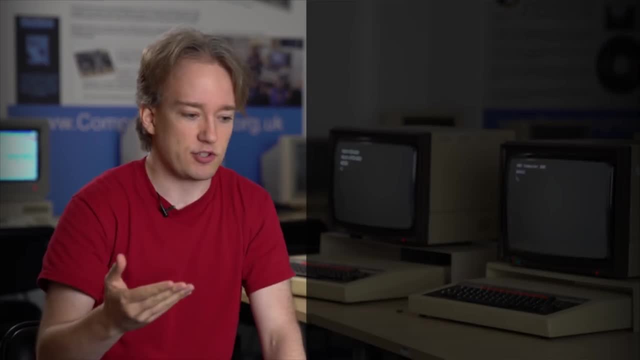 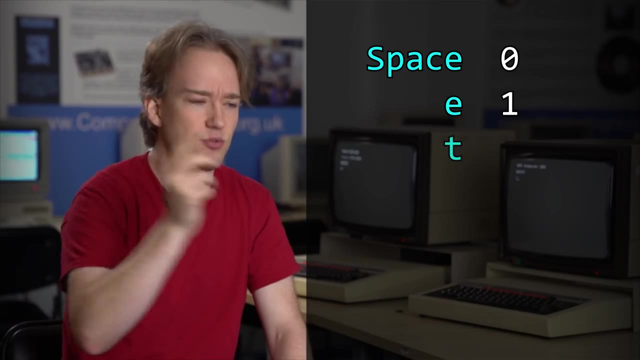 So those researchers way, way back could have said: well, the space bars generally used most often, just give that the code zero, Then it's the lowercase e. give that the code one, Then it's lowercase t, give that two zeros. 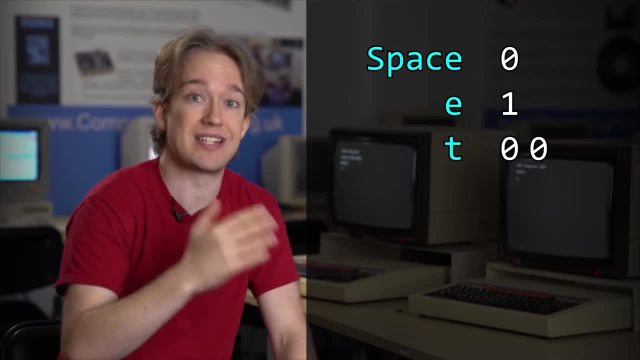 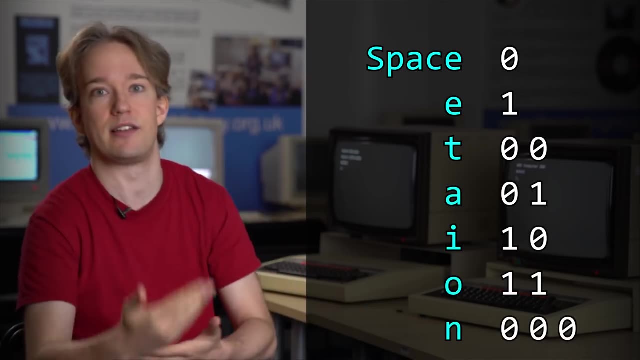 and immediately. we have hit a problem, Because the computer running through that text later has no way of knowing whether zero, zero is a t or the space bar twice. And if we keep on assigning letters like that, the problems keep getting worse. Is three zeros a lowercase n? 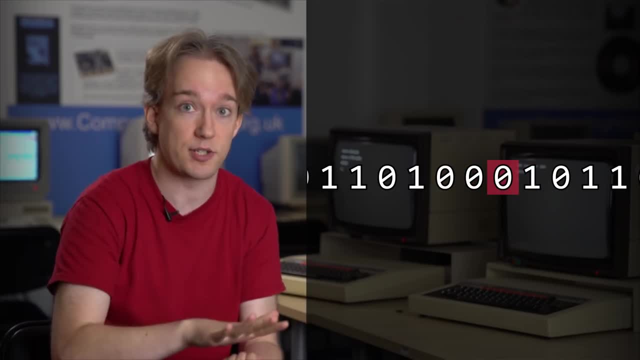 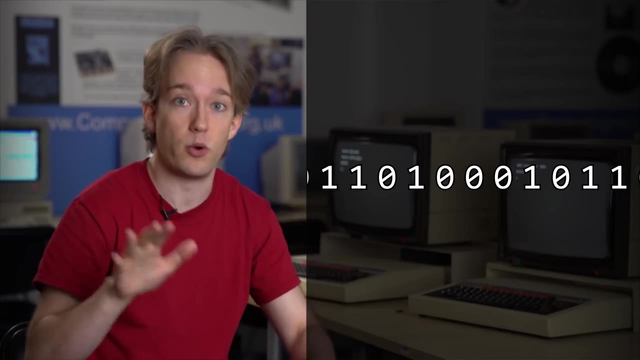 Or a t followed by a space, Or three spaces. Remember, there are no gaps here, no actual space separators. All the computer can see is a constant stream of ones and zeros. There's no way to know which is meant, Except in 1952, a very clever mathematician called David Huffman. 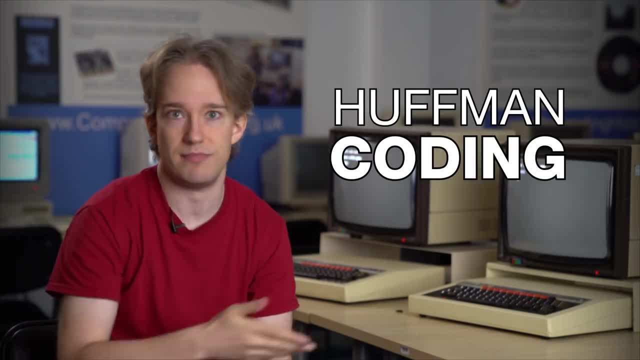 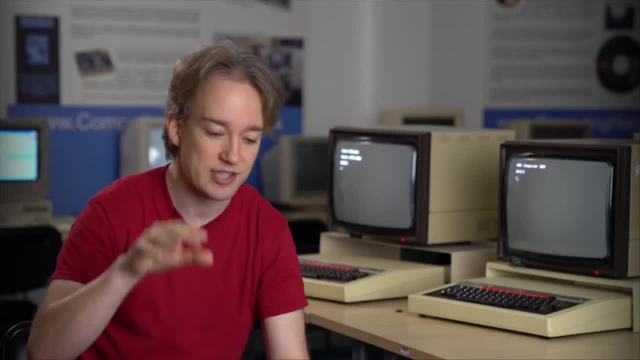 invented Huffman coding. You invent something like that. your name gets put on it. Yes, there are much better, more modern, more complicated mathematical ways to do this, but Huffman coding is the basic foundation of modern text compression, And here is how it works. 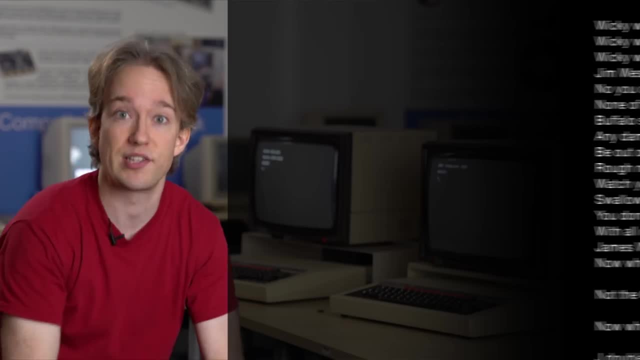 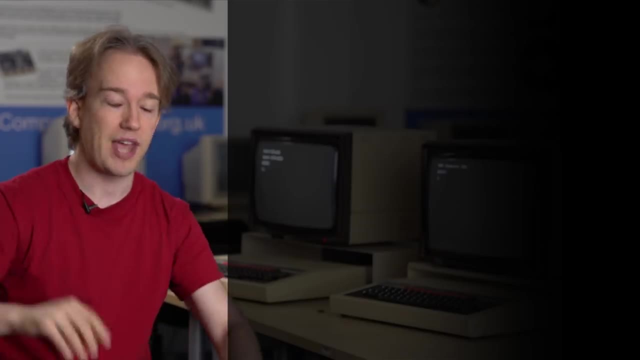 Let's say we want to compress. let's go with the lyrics to Will Smith's Wild, Wild West. Uncompressed, that is 3,684 characters taking up nearly 30,000 bits. First up, you count how many times each character is used. 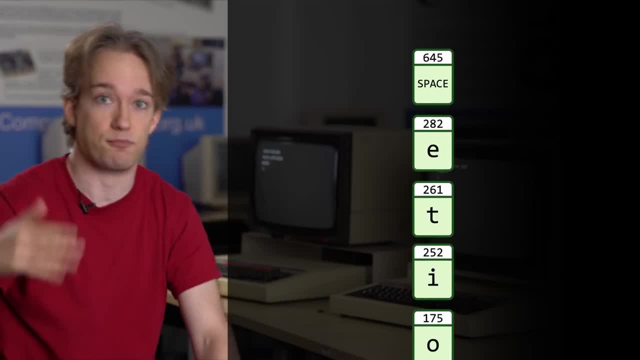 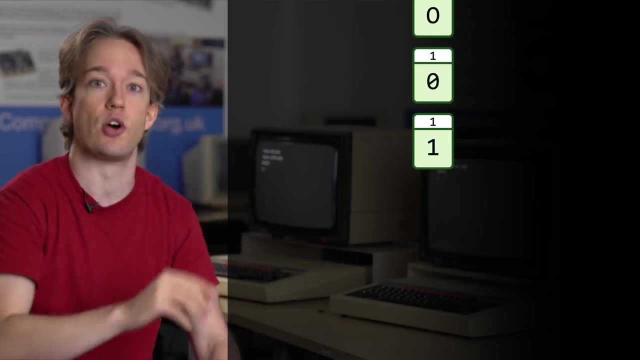 and you put that in a list in order. Now that'll be different for each block of text you're compressing. this has way more W's than usual. Now take the two least used characters. Those two are going to be the bottom branches on your Huffman tree. 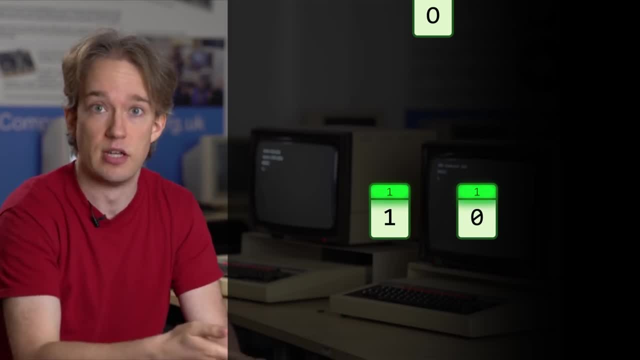 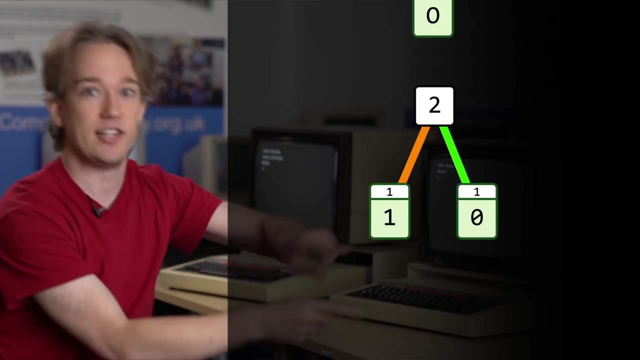 Write them down with how often they're used next to them. That's called a frequency. Then connect them together one level up with the sum of their frequencies. Now add that new sum back into your list wherever it sits higher up. 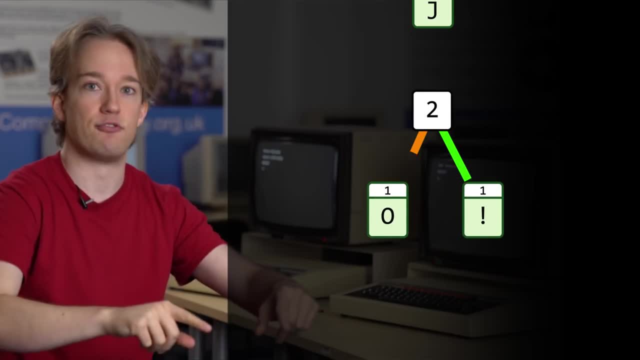 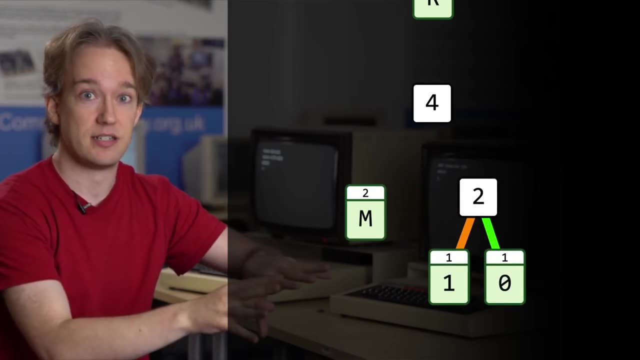 And repeat: Take the bottom two off your list, connect them up, add the result back into your list, keep that going And when one of the sums reaches the bottom two of the list, you connect it up. like that And eventually you are going to be down to. 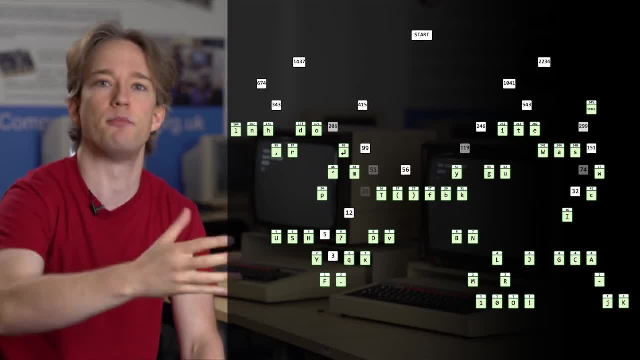 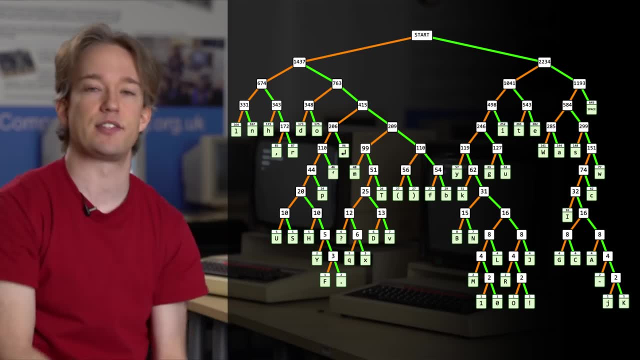 one thing: in your list right at the top, You now have a Huffman tree and it looks like this And it tells you how to convert your text into ones and zeros. Our first letter is the first uppercase W in wiki. wiki wild, wild west. 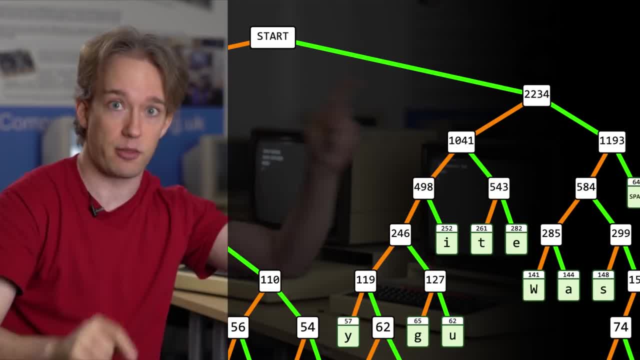 Uppercase W is here. there's 141 of them, so go to the top, follow the path down. Each time you take the left-hand side, write a zero. Each time you take the right-hand side, write a one. 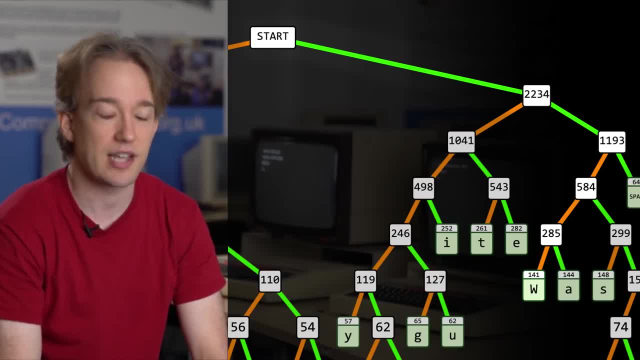 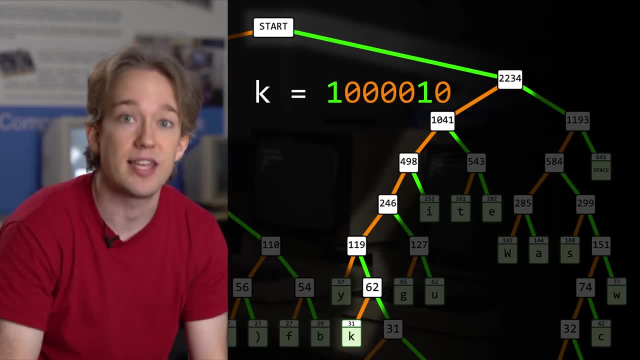 So W? is this? only five bits instead of eight. Next lowercase, i follow the code down: only four bits this time, Because it's more common than the K, which is less common. that actually takes up seven bits and you keep going. 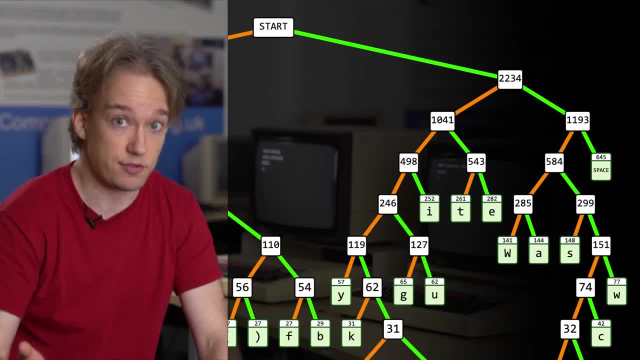 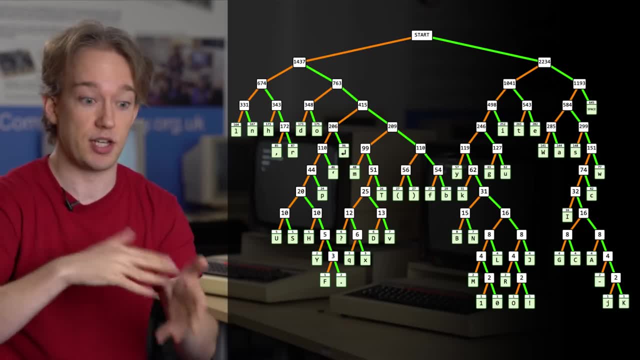 Some of the letters will take up more than eight bits, but that's fine, because they're not used very often. Now you do also have to store this tree to provide a translation table between your new symbols and the uncompressed ones, so this is not efficient for short bits of text.